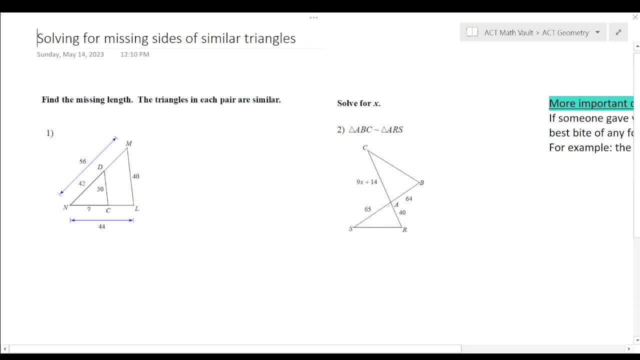 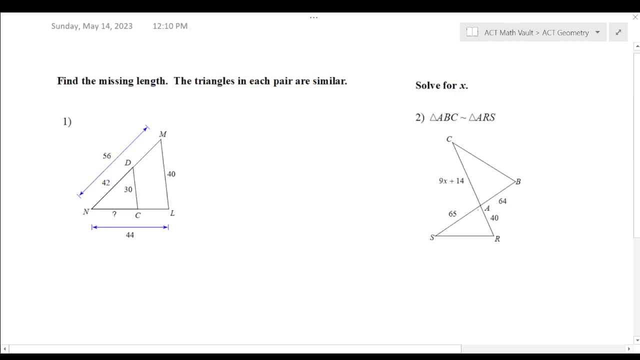 those look like. Well, these two are what I've seen most commonly, So you either have to solve for a missing side altogether or for a variable Within an expression that represents a side. All right, When a lot of students see this type. 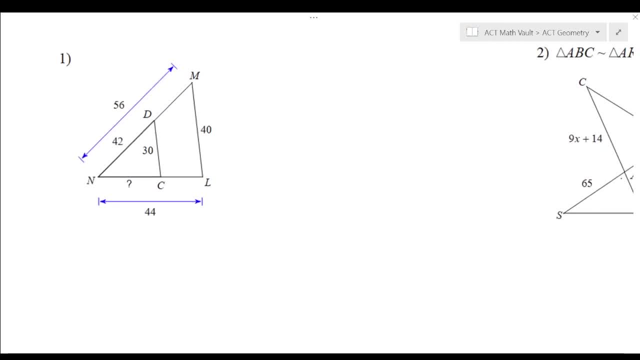 of a diagram. sometimes it's hard for them to tell that this is actually two triangles in one diagram, And so what I recommend for making sure you really get similarity straight is drawing out- and it does not have to look nice, but drawing out- two triangles. 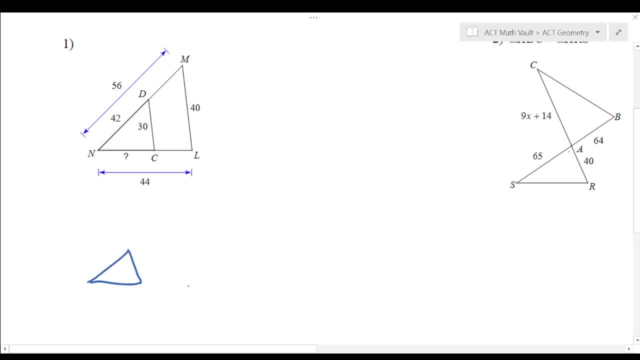 one that's smaller, one that's larger, Okay, And I know this is 42.. I know this is 30. And I'm solving for this side. on the smaller, It tells me that this is 56,, 40, and 44.. 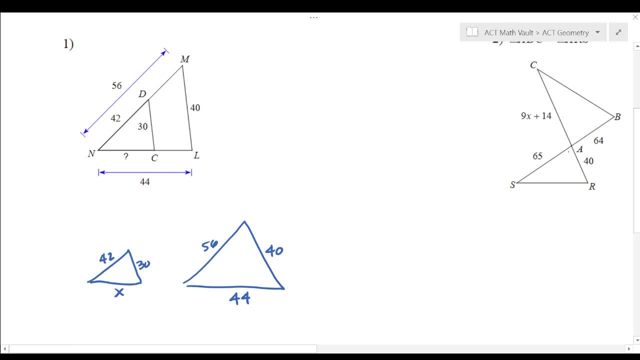 So right away I can tell in my diagram that there is- see this, 30 to 40, that's a three to four ratio of similarity. So I can tell that there is a three to four ratio of similarity And I can from the smaller to the larger. So what we can do is set up this x over 44.. Notice I'm doing smaller. 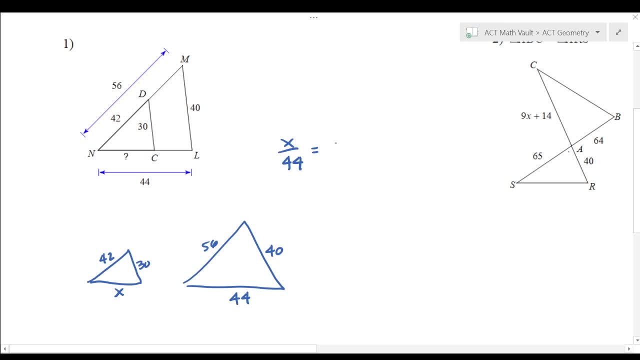 over larger And let's do the 30 and the 40. Just easier numbers to deal with. I also could observe that that simplifies to three fourths and set it equal to three fourths instead Doing a little mental math. 42 over 56 does simplify to three fourths And so it seems consistent And 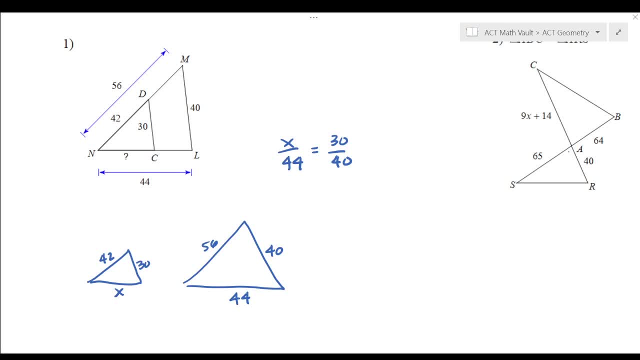 I'm also going to let it go here that we're really quickly doing this with the menu. Again, we have a little bit of delay, So you could think of what are we doing? I don't have to do the math here. I didn't start the math yet. And then we're just going to do it for the first time. So before we get into the math part, if we're going to be doing the math, we need to ask for a real quick calculation before we start the math. And we're going to start the math. 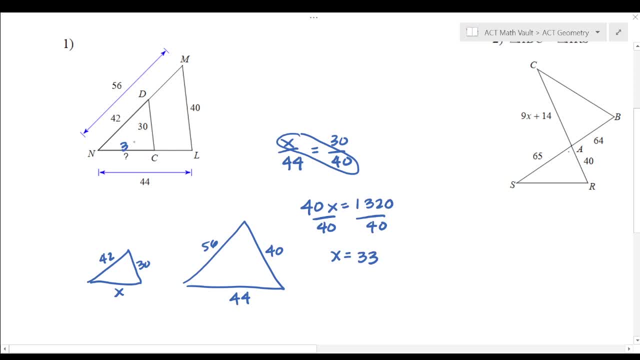 So we're going to start with the math, which is 40 to 40. And we're going to start with the math. So we're going to start with the math And then we're going to start with the math. 33, as this length right here. So that's the length of the whole thing. We called that length. 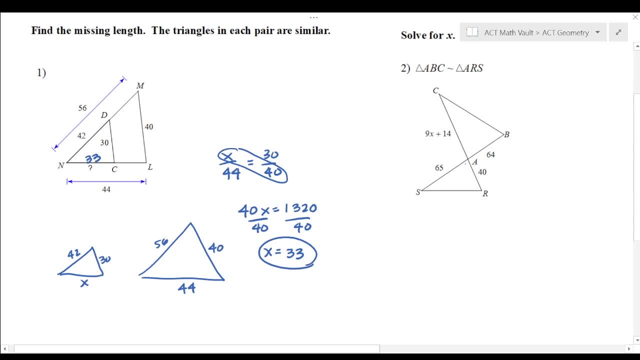 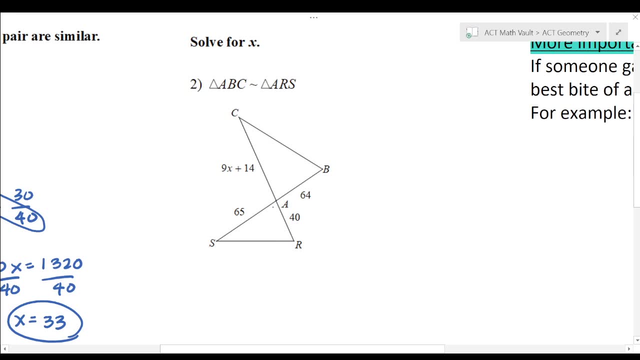 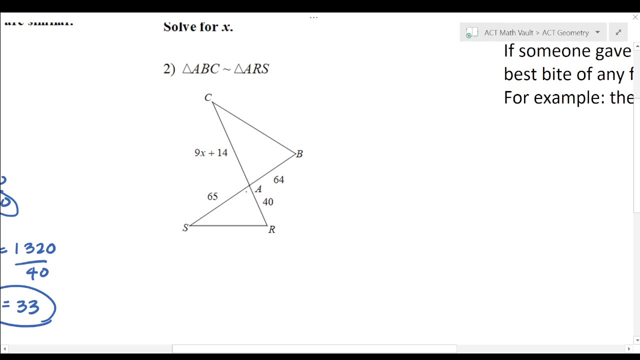 x here, But you could call it really whatever to be able to solve for. So let's move on to the next one. We have two triangles, And this one's a little bit harder because you can't really tell which segments line up with which for the proportion, until I think you draw those diagrams. 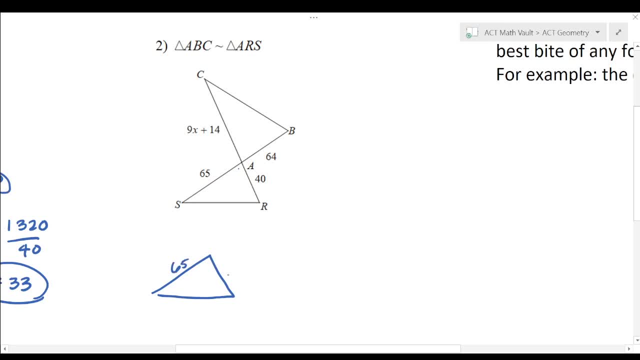 again. So we have the smaller 6540.. We have the larger, And this is where people start to go wrong, So we have to be really careful. It says ABC is similar to ARS And typically they'll give you that similarity statement. 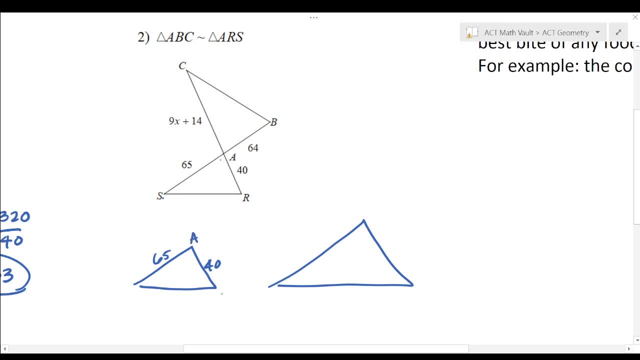 Because you need to know that ARS. ARS is similar to A, B, C. they go in the same spots, right? So A with A, B with R and C with S. Okay, so that means that this AB is this segment, right. 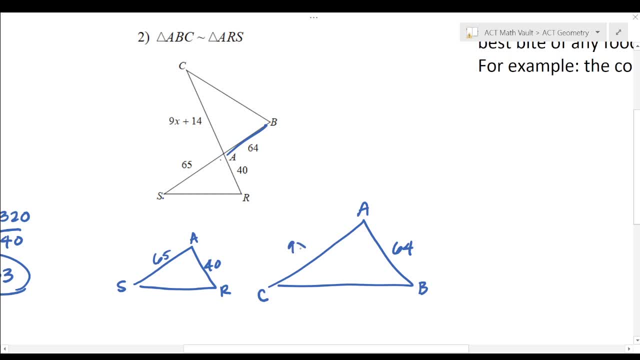 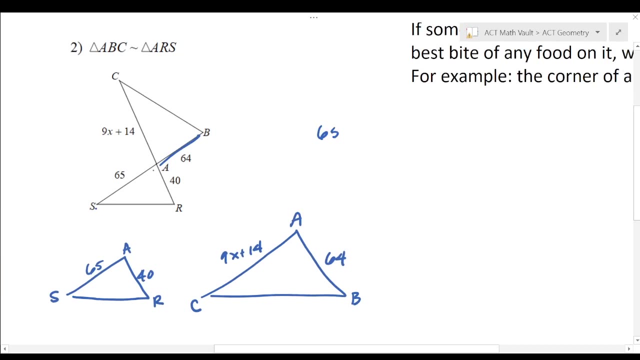 there 64. And then AC nine x plus 14 goes here. So now I can set up my proportion. it's clear as day that this will go with this right. Let's do small to big again with our ratio, So 65 over nine x plus. 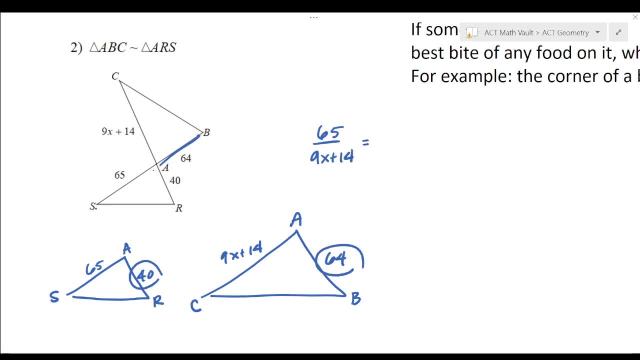 14 equals, and then small to big again, so 40 over 64.. Now keep in mind that a calculator will speed this up for you. Okay, that's 65. This is 65 times 64 equals, and then 40 times 64. And then: 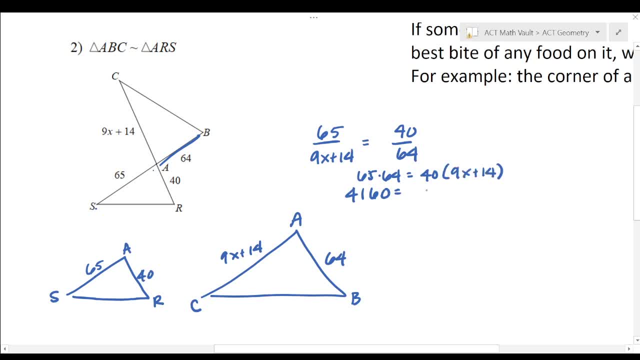 this is times nine x plus 1440. times nine x is 360 plus. and then I'm doing mental math. I'm thinking: 14 times 450, 650 plus zero. okay, then minus 5560 on both sides And we can just drop.